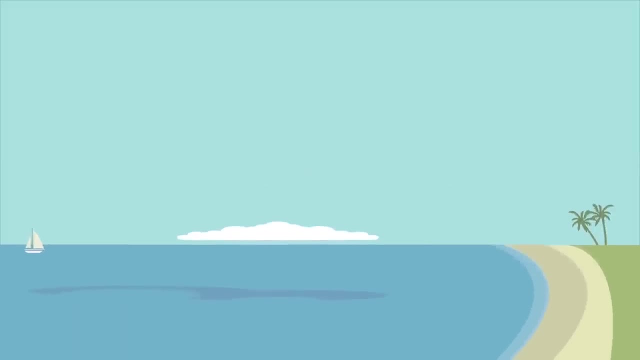 What causes sea level rise. If you've been to a beach before, you've probably noticed a sort of line where the ocean water meets the land. Of course, ocean water doesn't stay at the same level all the time. Waves and tides cause the level of the water to rise and sink all day long. 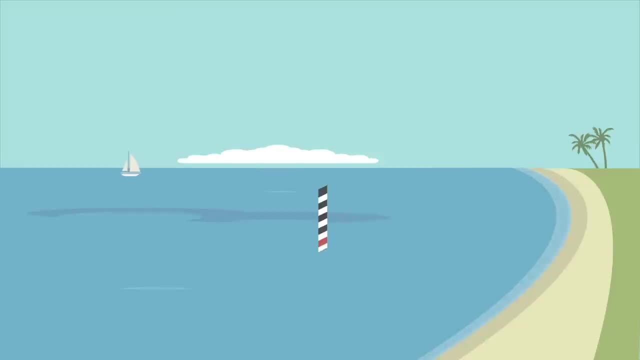 But we can measure the height of ocean water many times a day and figure out the water's average or typical height. The average height of the ocean in a particular place is called the local sea level, But the ocean covers most of our planet so it's way too big to measure with just a ruler. 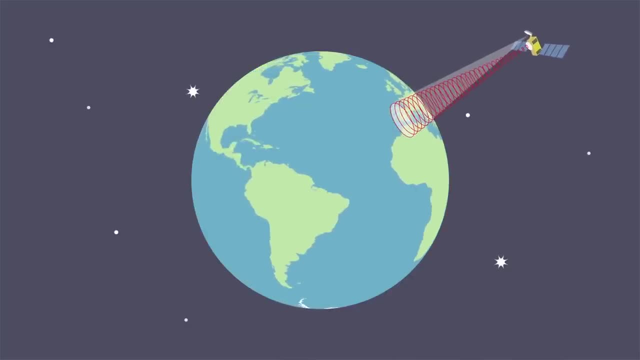 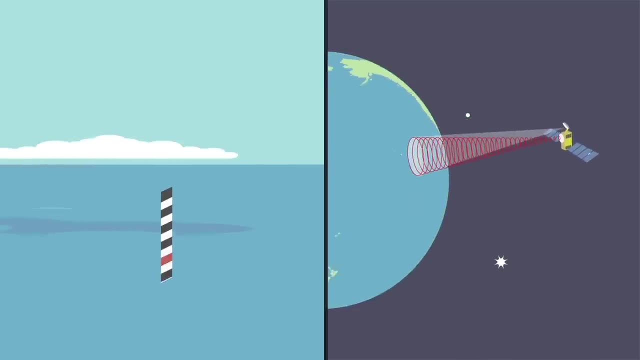 NASA measures the average sea level of the whole ocean from space. This measurement is called the global sea level. People have been measuring local sea level at certain times of the year. NASA has been measuring the global sea level for almost three decades. Over this time, scientists have 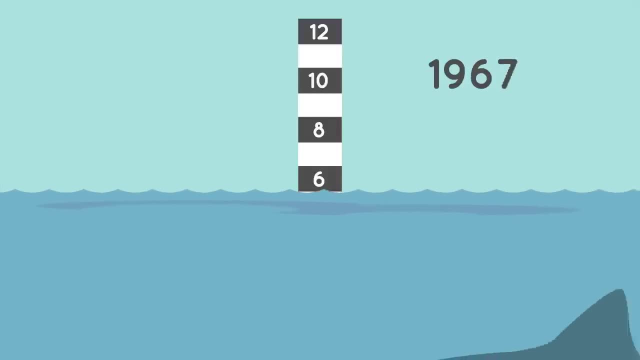 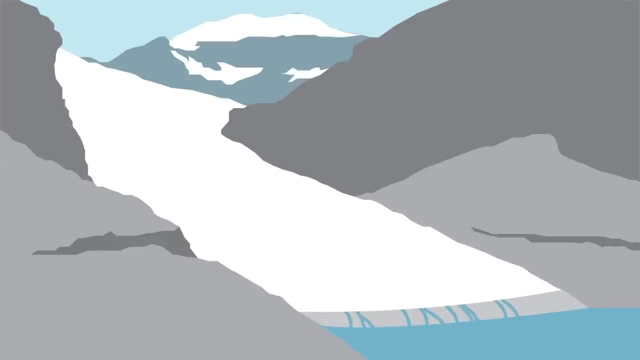 observed that the global sea level has been rising. The ocean is about seven to eight inches higher now than it was a century ago. Why? Because Earth is getting warmer. Glaciers and ice sheets are large masses of ice that sit on land. The ocean is a large mass of ice that sits on land. 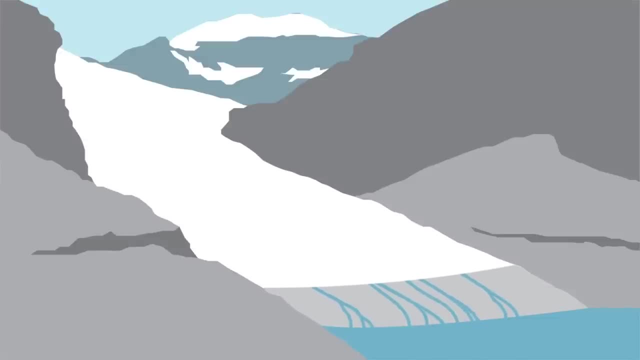 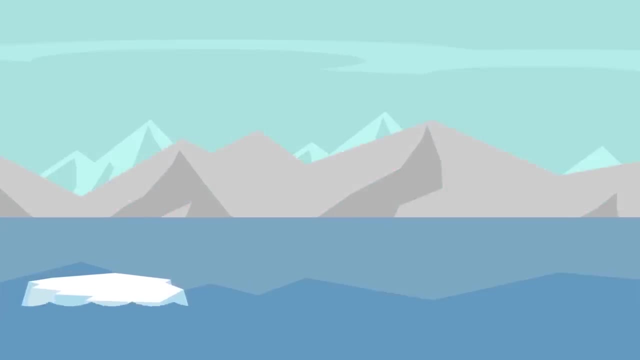 As our planet warms, this ice melts and flows into the ocean. More water in the ocean makes the sea level rise higher, But that's not the only way seas are rising. As Earth warms, the ocean is warming too. Water expands as it gets warmer, so warm water takes up more room in the ocean. 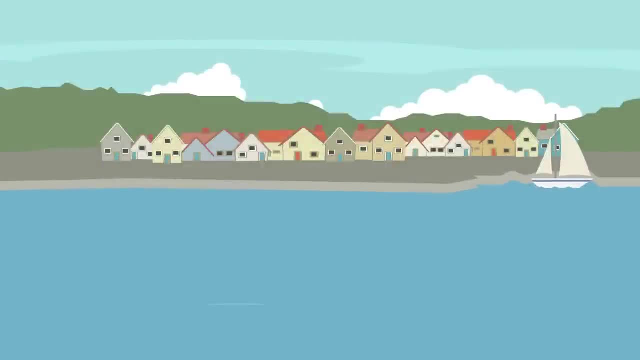 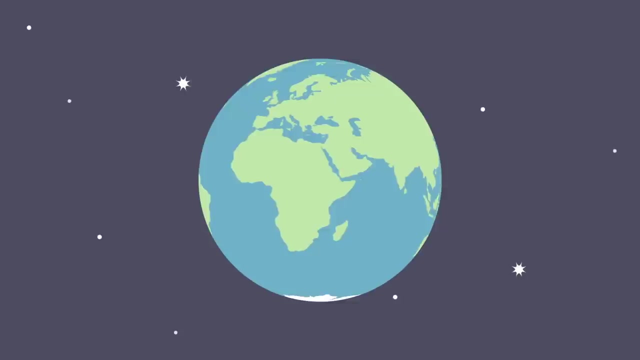 making sea levels higher. Rising sea levels can have an impact on how we live, especially in communities near the coasts. NASA and its partners use the Jason satellites to measure global sea level. It takes approximately 10 days for the satellites to complete one measurement.